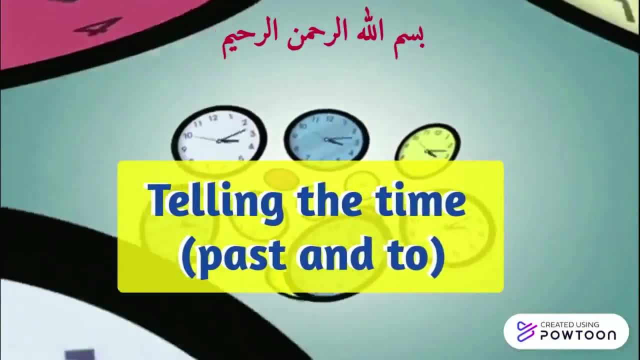 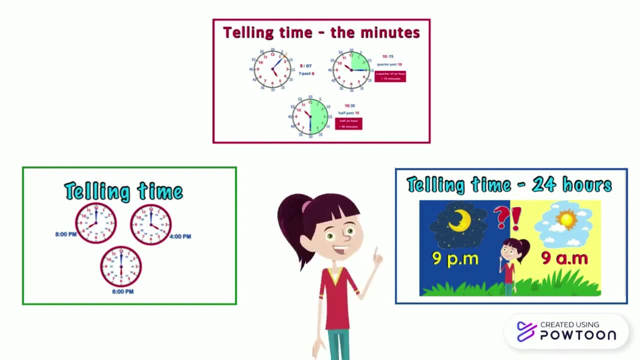 In this video we will learn how to tell the time using past and to. We have already seen in other videos how to read full hours, minutes and time in 24 hours, and in this video we are going to learn how to read the clock, but in a different way. 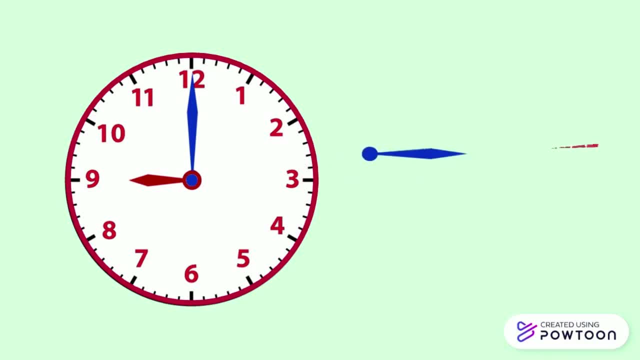 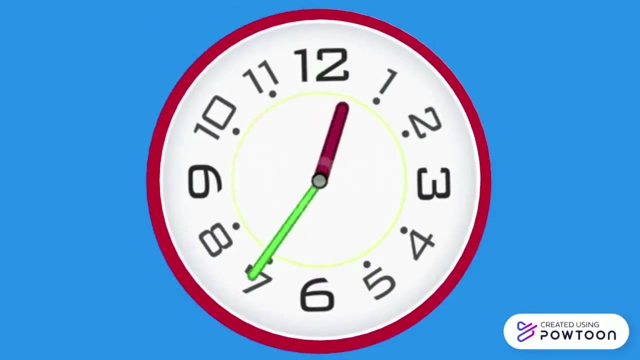 First of all, I will remind you that the big blue hand shows the minutes and the little red hand shows the hours And we have learned that on the clock face the minutes skip count 5 by 5.. Also, we have already said that the large hand goes around the clock face 60 minutes in one hour. 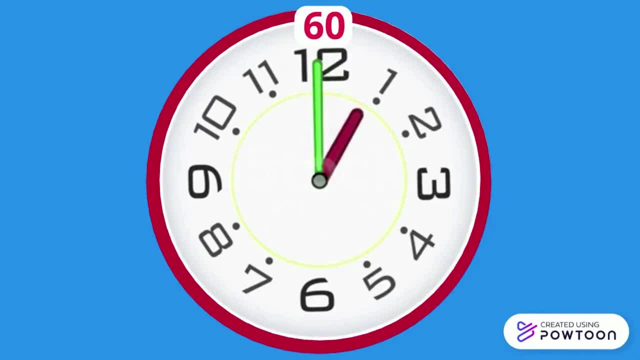 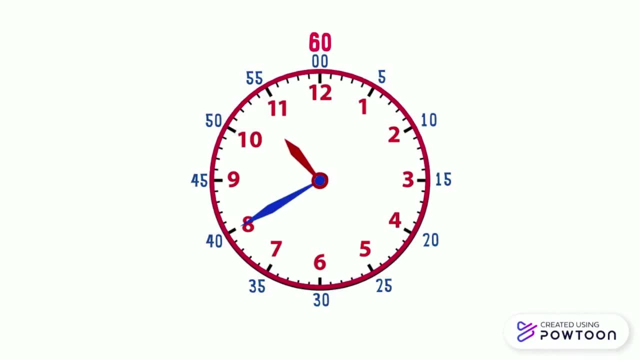 So let's write 60 above the 12 in order not to forget it. And of course, we start to read the hours first, then the minutes. For example, here it is 10: 40. But there is a different way to tell the time. We will learn how to read the hours first, then the minutes. For example, here it is 10: 40. But there is a different way to tell the time. 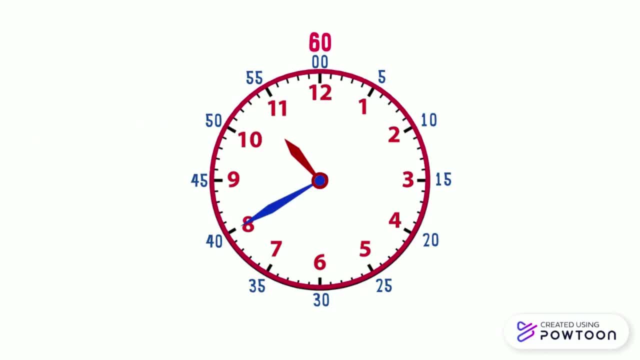 Let's find it out. The minute hand is not yet on the number 12, it's on the number 8.. So it's 40 minutes and we still need 20 minutes to go back up to the number 12, which represents 60 minutes. So pay attention. 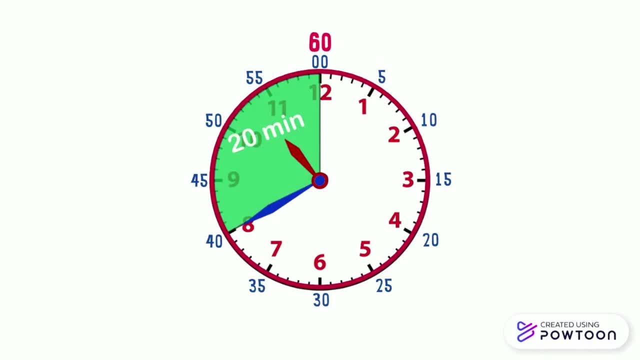 when the number of minutes is more than 30, which is more than half an hour, the time is closer to the next hour. So in this case we say the number of minutes remaining till the next hour. So we subtract our number of minutes from 60. So 60 minus. 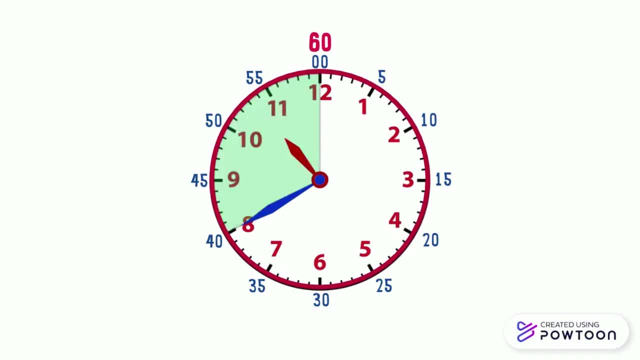 40 equals 20.. When the large minute hand moves 20 minutes, it will be back up at the number 12 and the small hour hand will be at the number 11.. So 10: 40 is also 20 minutes to 11. 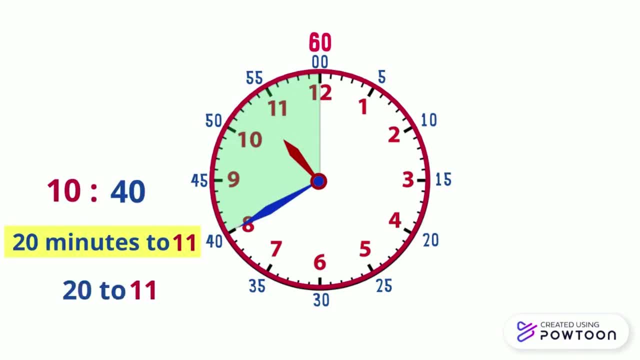 which means it still needs 20 minutes to be 11 o'clock. Here it is 2: 50 and there are 10 minutes left to be 3 o'clock. So it's 10 minutes to 3, or we can say 10 to 3.. So we should figure out how many minutes that the minute hand needs to move to the next. 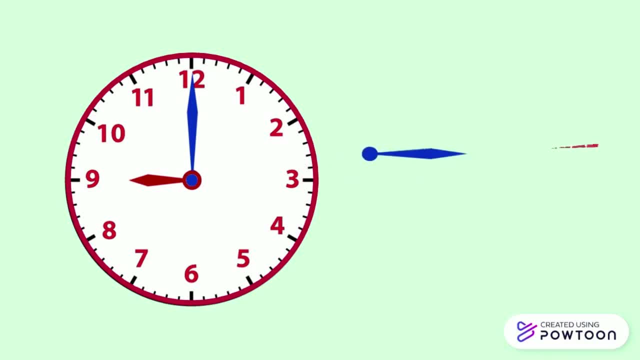 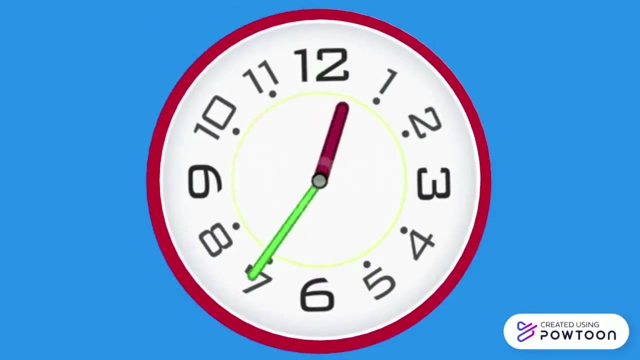 First of all, I will remind you that the big blue hand shows the minutes and the little red hand shows the hours And we have learned that on the clock face the minutes skip count 5 by 5.. Also, we have already said that the large hand goes around the clock face 60 minutes in 1 hour. 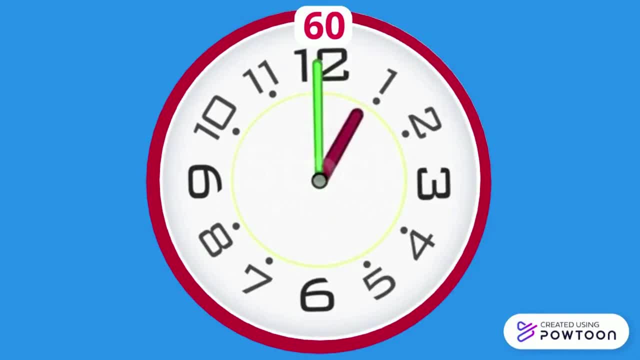 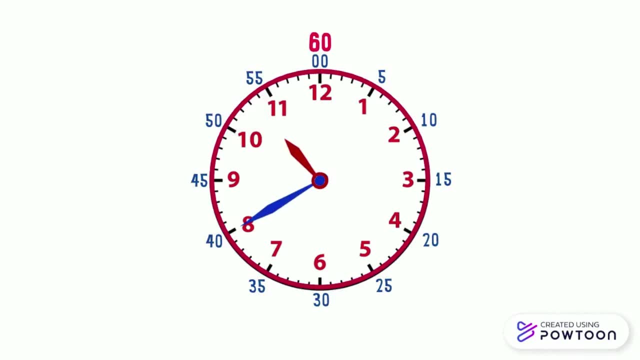 So let's write 60 above the 12 in order not to forget it. And of course, we start to read the hours first, then the minutes. For example, here it is 1040.. But there is a different way to tell. the time. First of all, we will learn how to read the hours first, then the minutes. For example, here it is 1040.. But there is a different way to tell the time. First of all, we will learn how to read the hours first, then the minutes. For example, here it is 1040.. But there is a different way to tell the time. 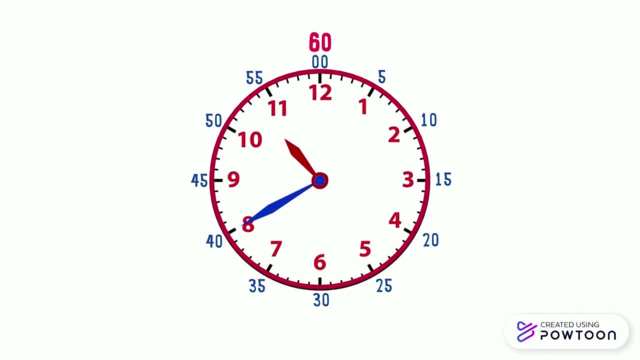 Let's find it out. The minute hand is not yet on the number 12,, it's on the number 8.. So it's 40 minutes and we still need 20 minutes to go back up to the number 12, which represents 60 minutes. So pay attention. 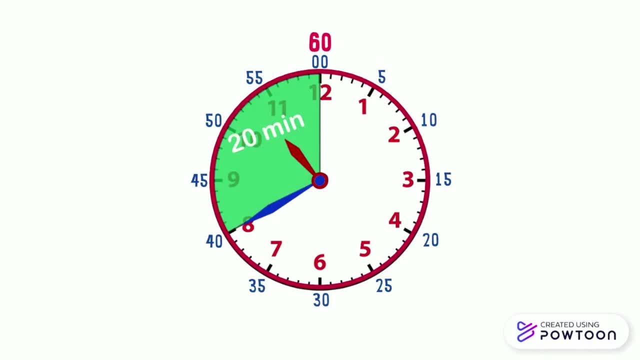 when the number of minutes is more than 30, which is more than half an hour, the time is closer to the next hour. So in this case we say the number of minutes remaining till the next hour. So we subtract our number of minutes from 60.. So 60 minus. 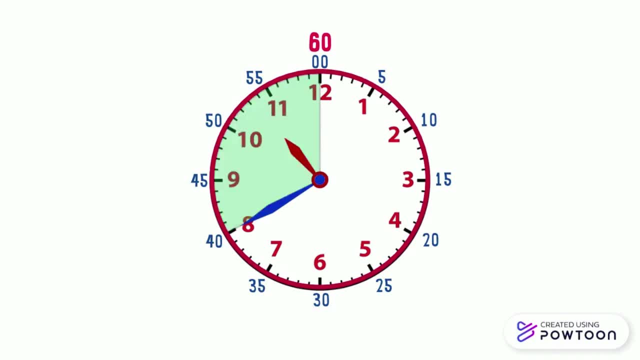 40 equals 20.. When the large minute hand moves 20 minutes, it will be back up at the number 12, and the small hour hand will be at the number 11.. So 1040 is also 20 minutes to 11,. 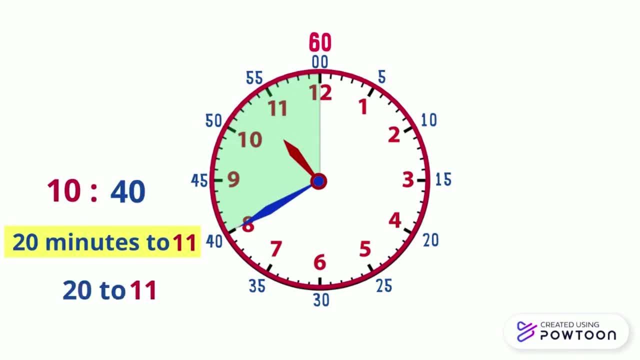 which means it still needs 20 minutes to be 11 o'clock. Here it is 2.50, and there are 10 minutes left to be 3 o'clock. So it's 10 minutes to 3, or we can say: 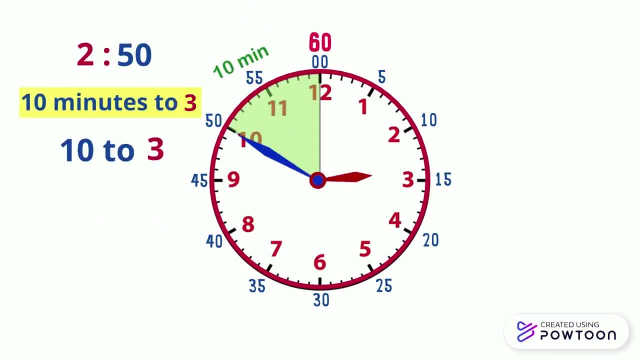 10 to 3.. So we should figure out how many minutes that the minute hand needs to move to the next whole hour. Another example: here it is 6.55, and there are 5 minutes left to be 7 o'clock, So it's.